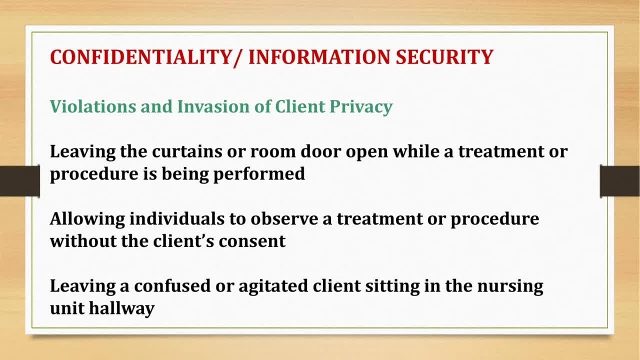 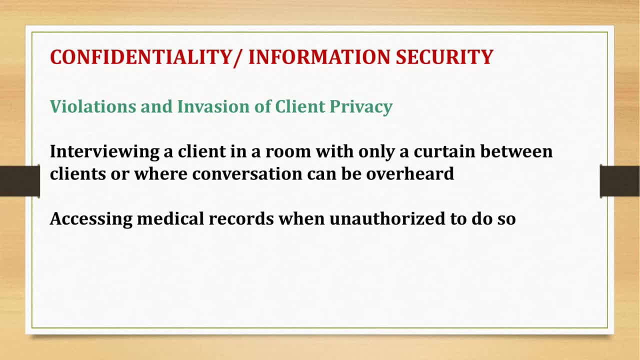 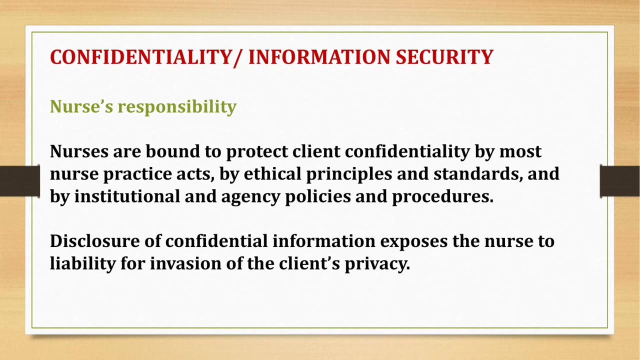 client sitting in the nursing unit hallway, interviewing a client in a room with only a curtain between clients or where conversation can be overheard, accessing medical records when unauthorized to do so. Nurses are bound to protect client confidentiality by most nurse practice acts, by ethical principles and standards, and by institutional and agency policies. and. 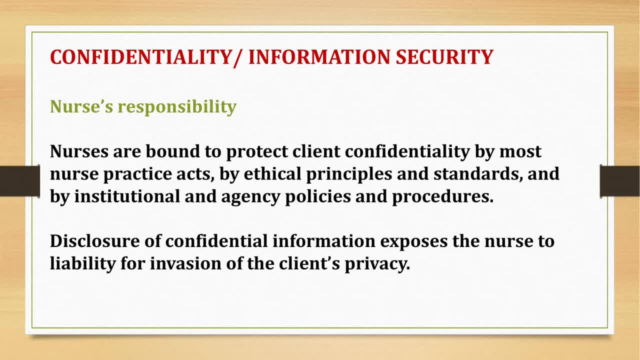 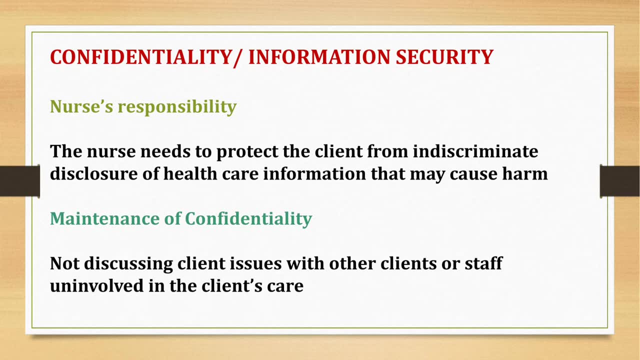 procedures. Disclosure of confidential information exposes the nurse to liability for invasion of the client's privacy. The nurse needs to protect the client from indiscriminate disclosure of health care information that may cause harm. Maintenance of confidentiality: Not discussing client issues with other clients or staff uninvolved in the client's care. 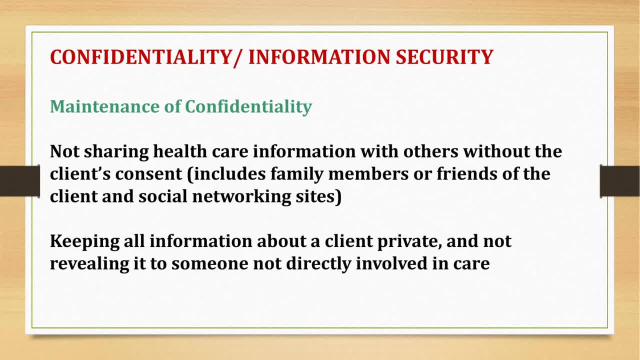 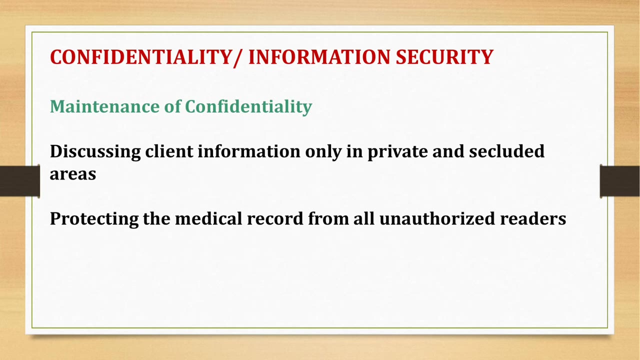 Not sharing health care information with others without the client's consent includes: family management. Keeping all information about a client private and not revealing it to someone not directly involved in care. Discussing client information only in private and secluded areas. Protecting the medical record from all unauthorized readers. 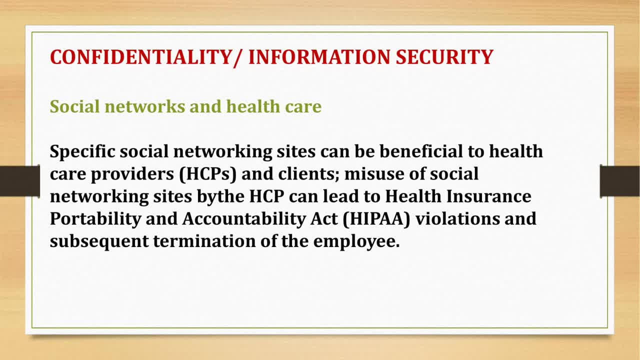 Social networking and health care. Specific social networking sites can be beneficial to health care providers, HCPs and clients. Misuse of social networking sites by the HCP can lead to Health Insurance Portability and Accountability Act, HIPAA violations and subsequent termination of the employee. 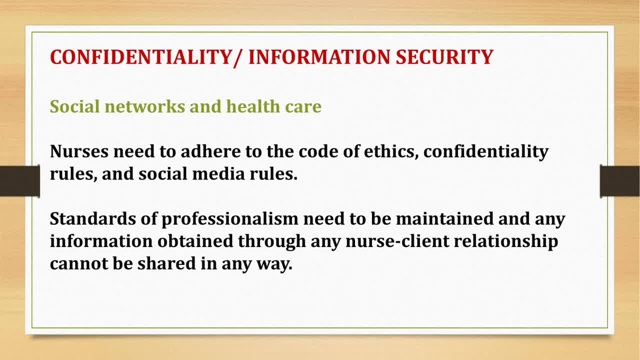 Nurses need to adhere to the Code of Ethics, Confidentiality Rules and Social Media Rules. Nurses need to adhere to the Code of Ethics, Confidentiality Rules and Social Media Rules. Nurses need to adhere to the Code of Ethics, Confidentiality Rules and Social Media Rules. 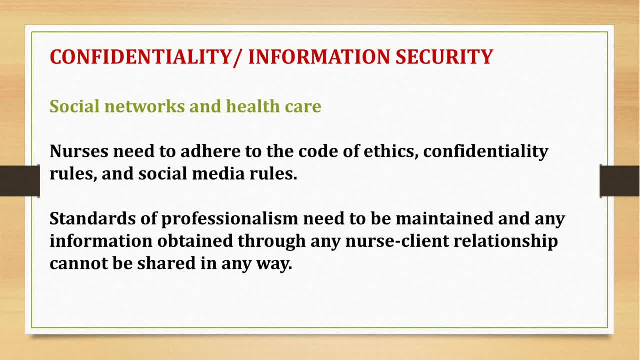 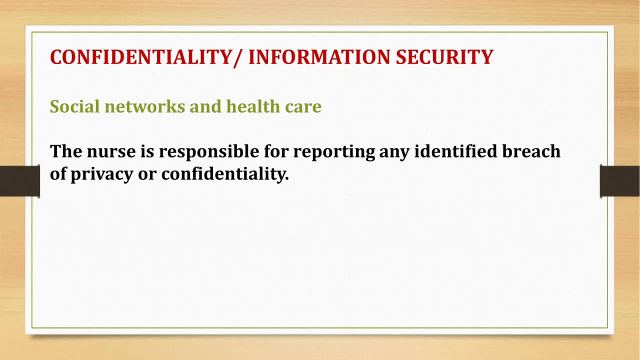 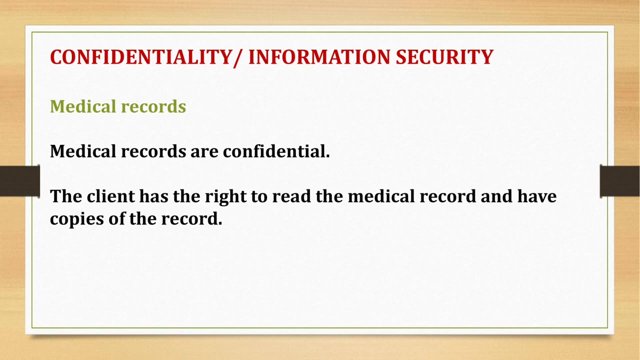 Standards of professionalism need to be maintained and any information obtained through any nurse-client relationship cannot be shared in any way. The nurse is responsible for reporting any identified breach of privacy or confidentiality. Medical records. Medical records are confidential. The client has the right to read the medical record and have copies of the record. 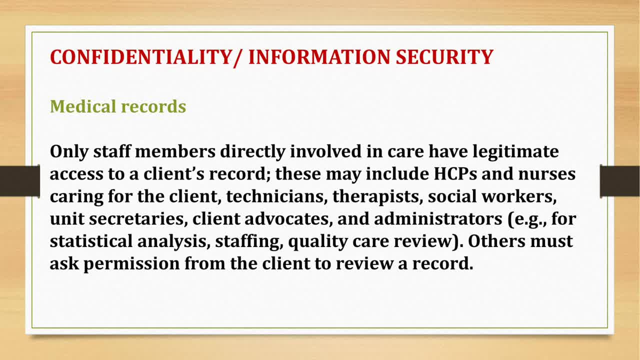 Only staff members directly involved in care have legitimate access to a client's record. These may include HCPs and nurses caring for the client, technicians, therapists, social workers, unit secretaries, client advocates and administrators. Example For statistical analysis. 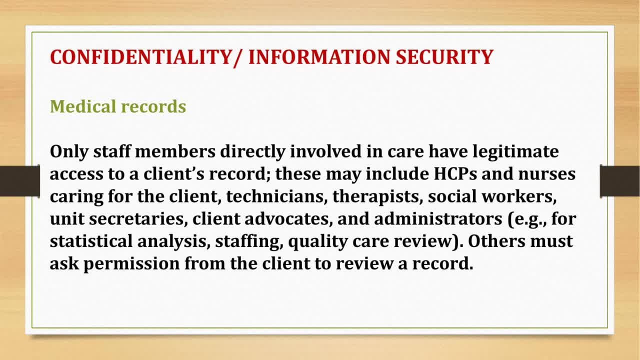 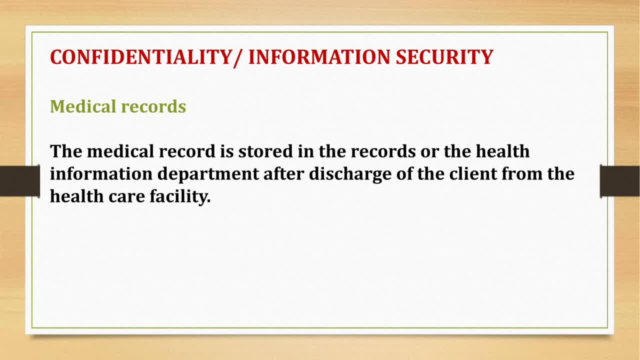 Staffing. Quality care review. Others must ask permission from the client to review a record. The medical record is stored in the records or the health information department after discharge of the client from the health care facility. Information technology slash- computerized medical records. 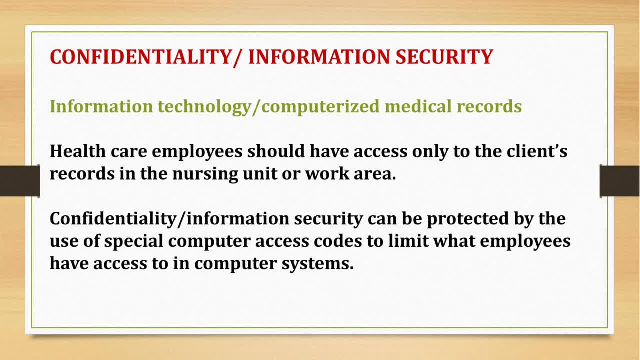